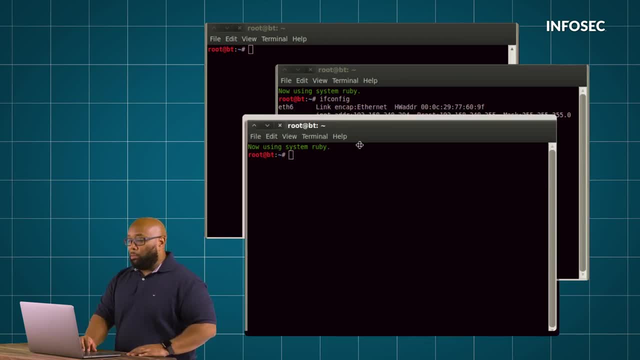 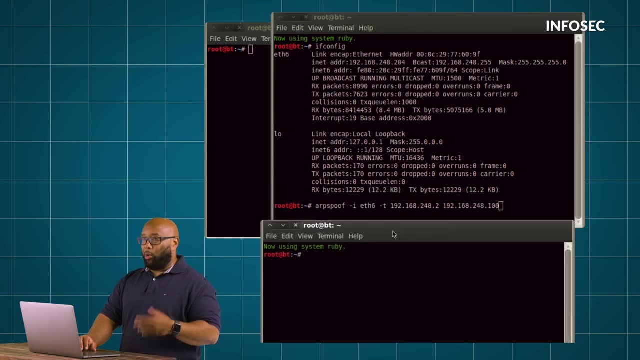 100.. Now for man in the middle to work. remember, you're in the middle or you're trying to get in the middle. so you can't just art poison one side of that equation, you have to art poison both. So now, simultaneously, I'm going to art poison and tell the gateway which, if you're at home or 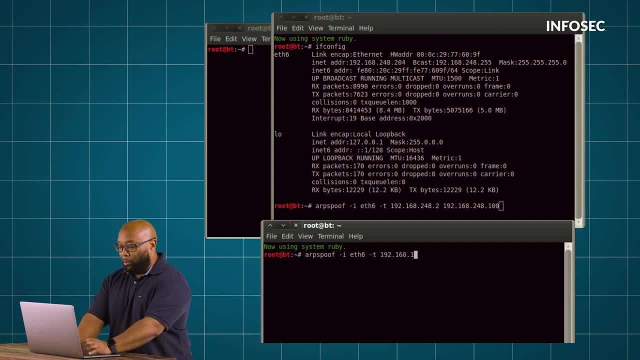 at Starbucks. this gateway would essentially be your wi-fi router that we're spoofing here. So now I'm going to tell the victim that I am the gateway. So first art spoof: I'm telling the gateway that I'm the victim. The second art spoof: I'm telling the victim that I'm the gateway. 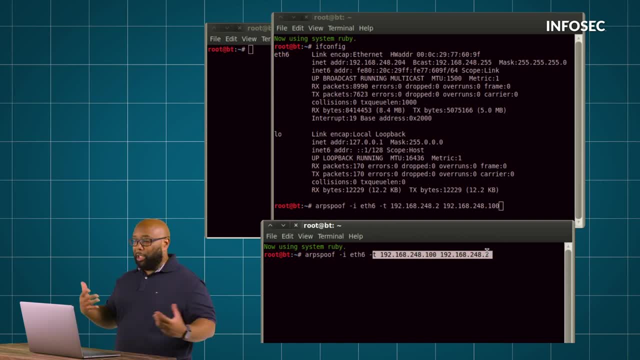 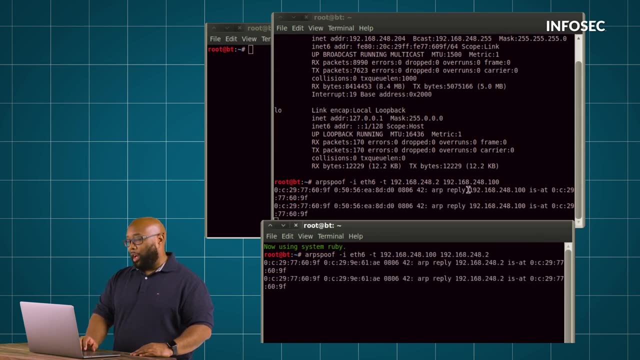 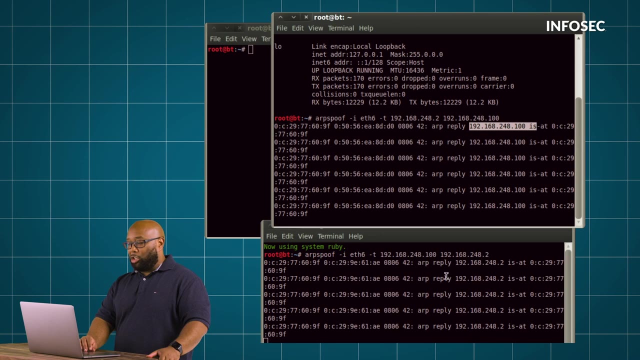 This is part of what puts me in the middle. Both sides will now think I'm the other side. So I start my art poison and right away you can see the art going out and it's doing a reply which is telling the 100 machine that I'm the gateway and it's also telling the gateway that I'm the 100 machine. 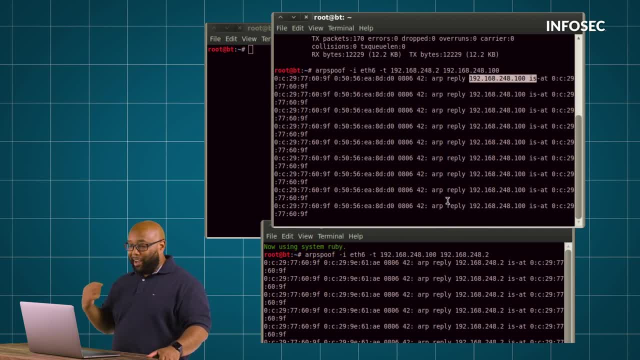 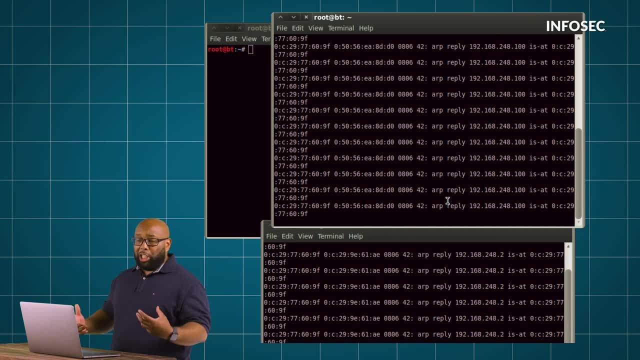 So that's the art poisoning in motion, and it's going every second. The reason it's going every second is because in a real network, every once in a while the real machines would respond and say: wait a minute, I've got that IP address. So having this art happen every second guarantees that even 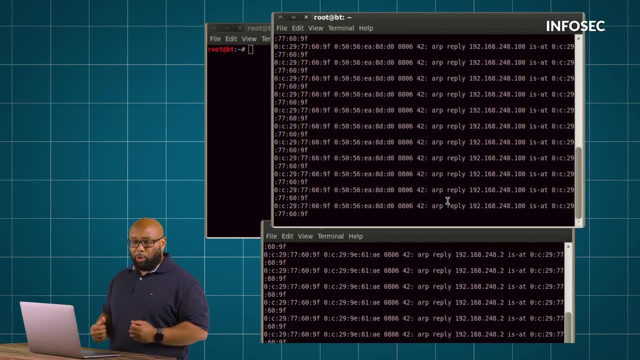 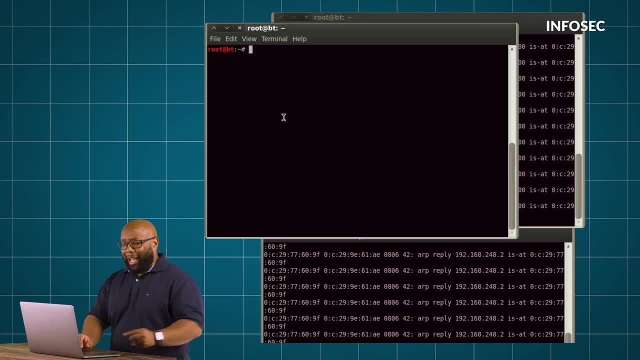 if the real device responds, you immediately overwrite that response with your more recent response, Because in the land of art the most recent reply is considered to be the truth. So the last step, once we've got the art poison going here, to set up the infrastructure is we? 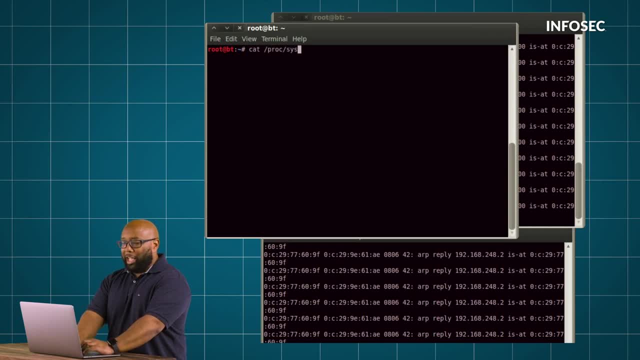 have to make sure we turn on something called IP forwarding, And the reason for that is: by default, your machine will simply drop packets. that's not going to be able to get to the IP address, So if it's not intended for it. Now, in my case, my machine has the IP for it turned off, which means 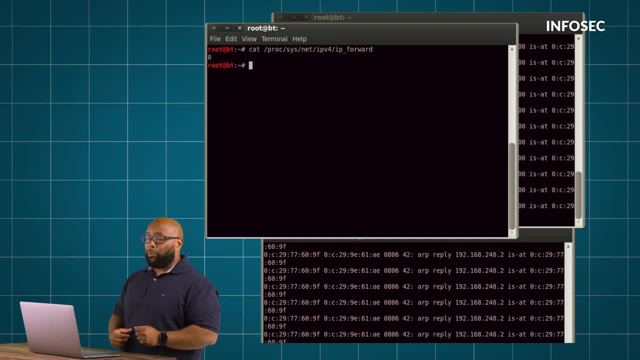 it's going to follow that behavior, and all machines do that by default. What I want to do is change that behavior, because I am going to be getting packets that are intended for our victim here, and since those packets aren't actually intended for me, my default behavior is to simply. 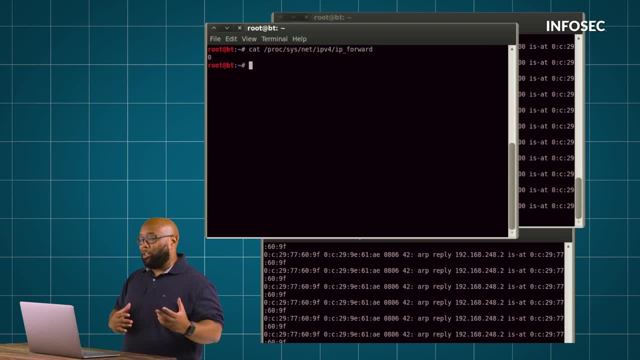 drop those packets. but I don't want to drop them. I want to go ahead and take them and pass them on. So I'm going to change this IP forward from a value of zero. to guess what, if it's zero is off, what do you think I need to change it to to turn it on? Exactly, you won one, so I'm 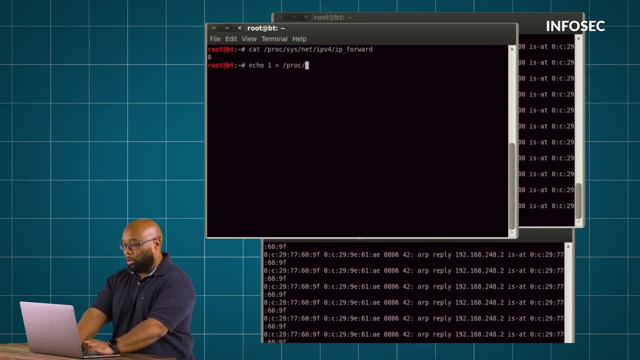 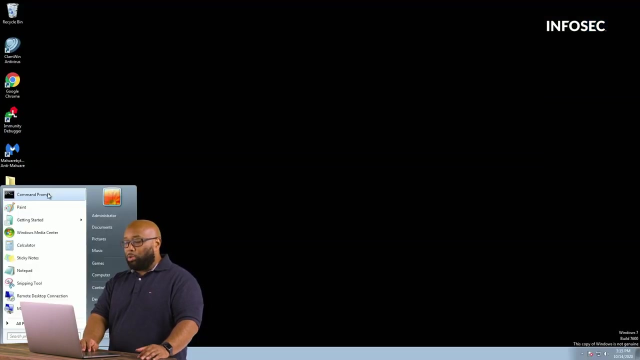 simply going to write the number one into this file, And this will actually turn on IP forwarding. Now, to prove to you that this is working, I'm not going to write this yet. I'm going to show you that currently, one hundred, which is, has trouble pinging dot two. 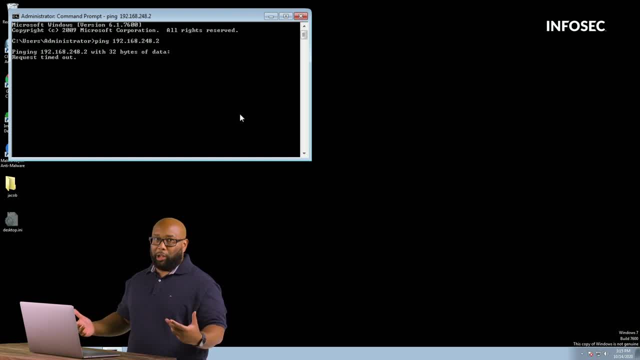 And that's because the ping packet is never making it to the actual gateway. it's coming to my machine and since my default behavior is a drop packets- not meant for me and I'm clearly not dot two that packets getting dropped- But the minute I turn on IP forwarding, 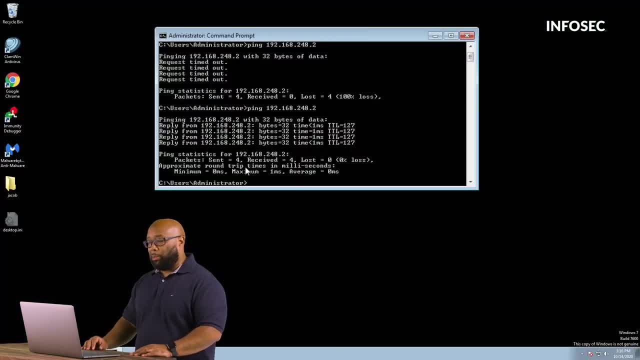 let's go ahead and turn that on. Now you're going to see, those pings are going to end up being 100% successful, And that's because now the ping is making it to the other side, but it's only making it there by coming through my interface first. So that means I've made myself a proxy, or now I've 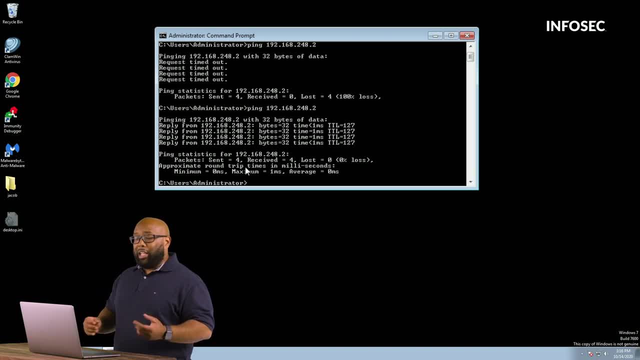 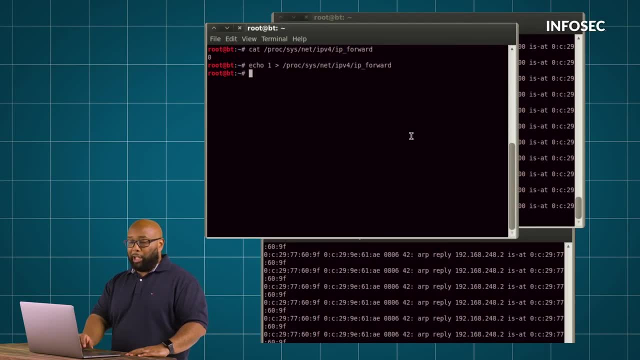 completed and put myself in the middle. All right, The next part. how do we prove that and how can we do things? Well, there's a couple of tools that I want to show you on top of us being in the middle. First one is a special purpose sniffer called DriftNet. What DriftNet does is it is unique in 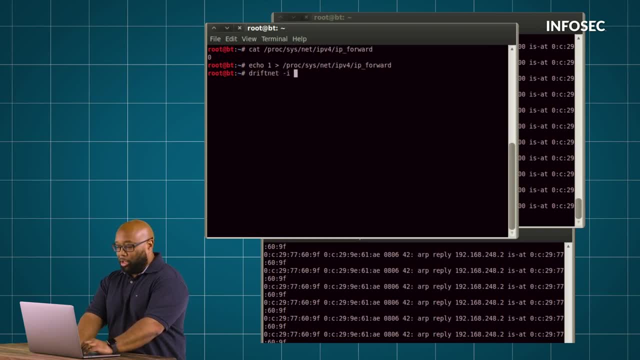 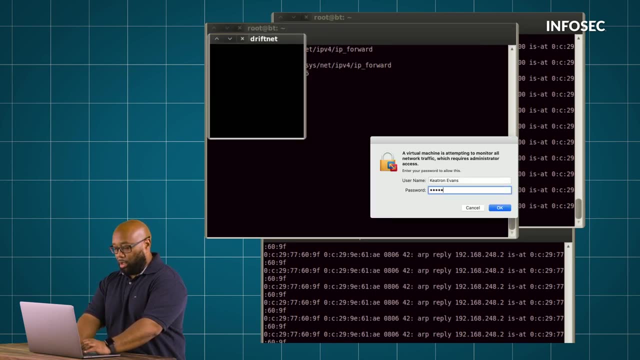 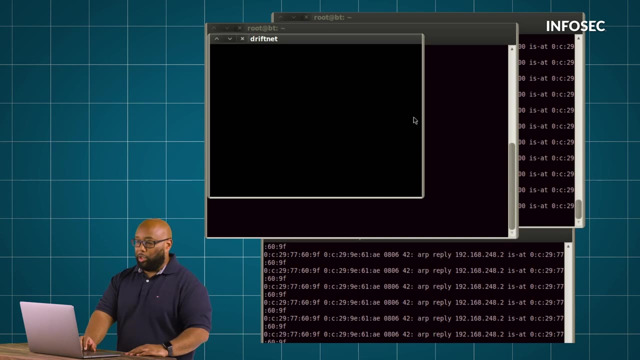 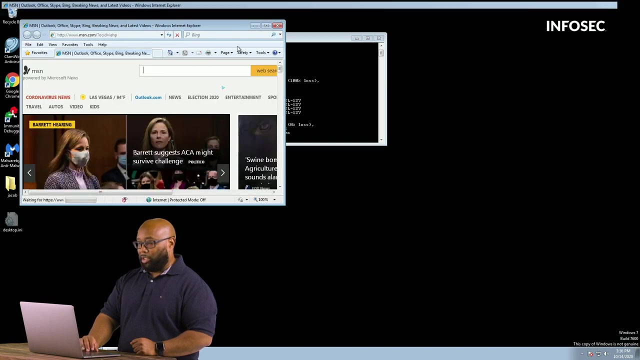 that it grabs only images out of a victim's traffic. So if I run DriftNet, tell it to listen on interface six here. What you're going to see in this little black window is whenever the victim visits websites, Let's go do that. Victim goes out, goes to MSN and some other places. 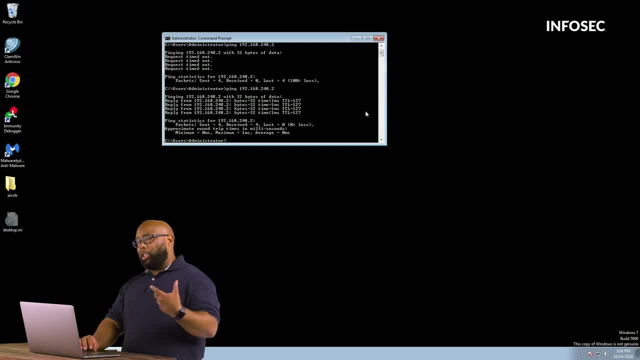 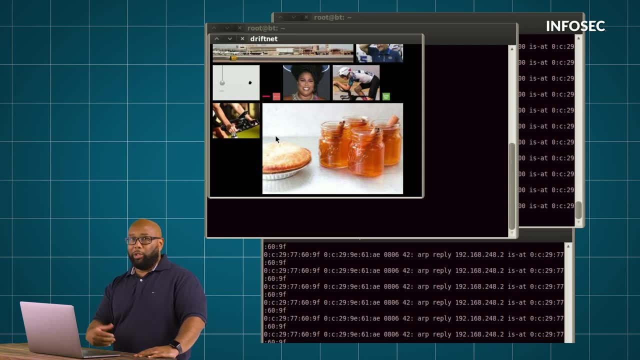 Well, in that traffic are images. Well, guess what the attacker just grabbed. All of the images that were in that traffic has now been sniffed off by this attacker who's in the middle. So any images that you would have viewed during your browser session, the attacker. 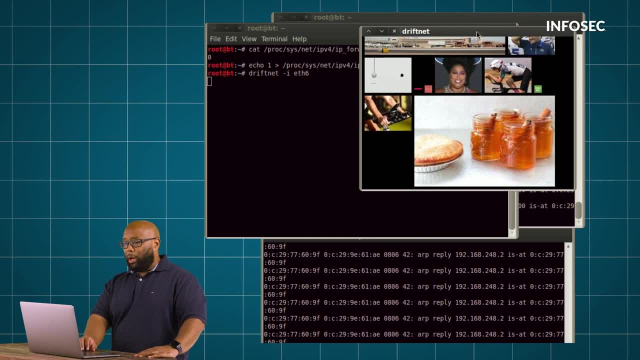 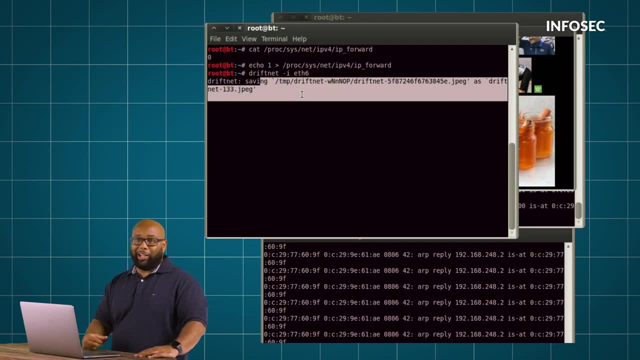 is able to see those images. now, Not only see them, but if I found one that I wanted to keep, like this image here with this nice pie, I click that and it actually saves a local copy of that image so that I can go back and look at it and view it later. Now, if that's not creepy enough, 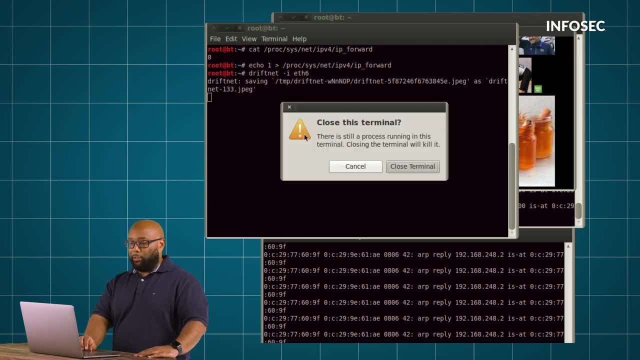 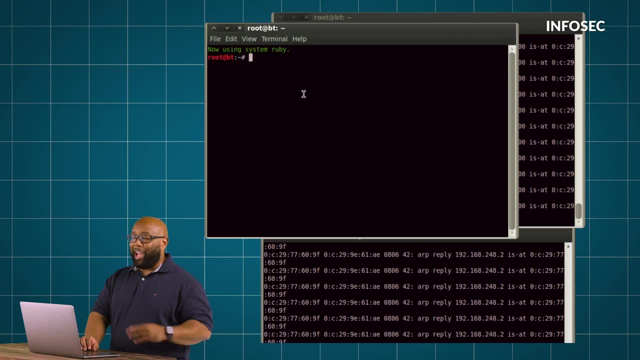 Let me show you how this really gets deep. So, on top of the man in the middle and on top of the art poisoning, I'm going to do one more thing, called DNS cache poisoning, And what this means is, whenever you go to a website such as Facebook, the first thing that happens is your machine sends: 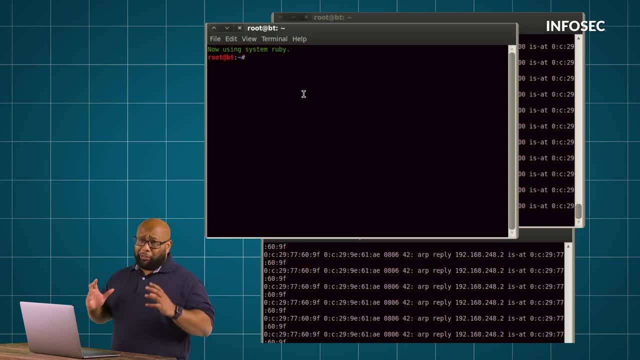 a query to your DNS server saying where is Facebook, What's Facebook's IP? Your DNS server responds back and says: here's the IP address for Facebook. Now what I'm going to do is, since I'm in the middle, I'm going to see that request and I'm going to respond on behalf of the actual DNS. 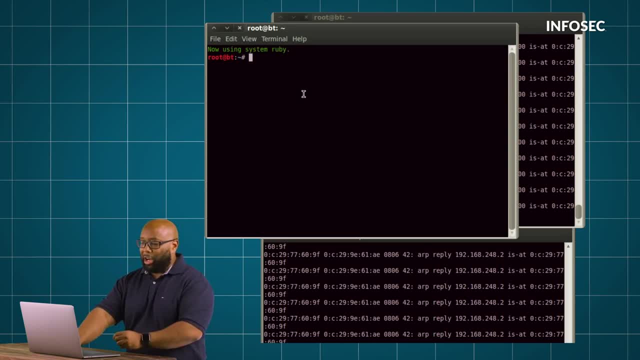 server and lie to you and tell you that Facebook is at my machine. Let's look at how easy that is. So I'm first going to create a file. We'll just call this MITM, FB for Facebook, and I'm just going to say in there that Facebook. 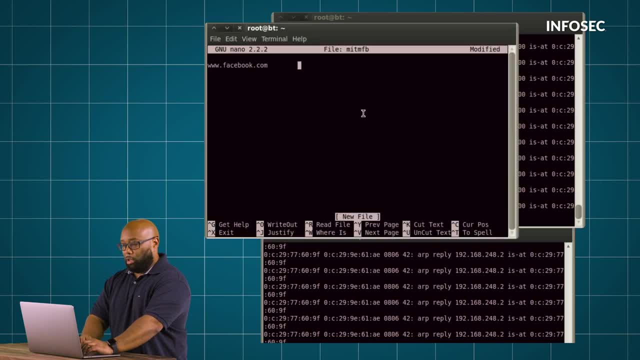 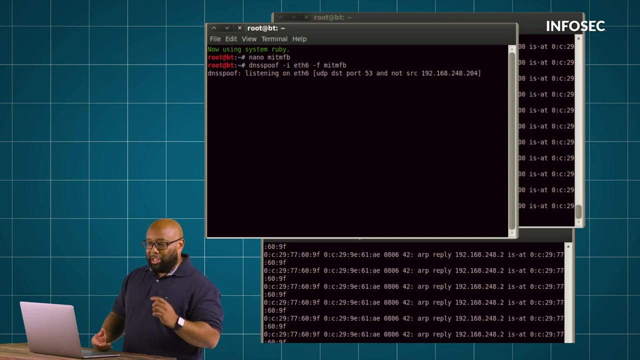 is at my IP, which is 204.. And then I'm going to call my server as well, Save that little text file. And now I'm gonna run the tool DNS spoof Point to that file that we just created. And now what's happening is: anytime this tool sees a query for Facebook, it's gonna respond to that. 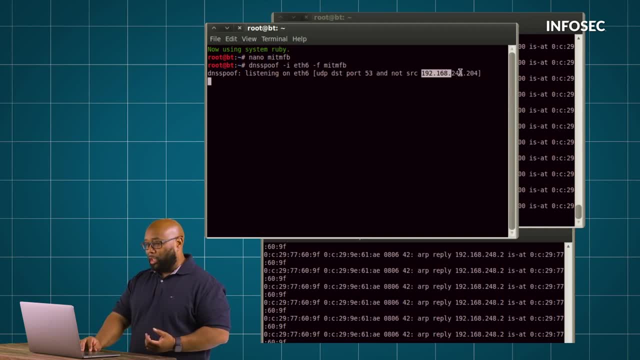 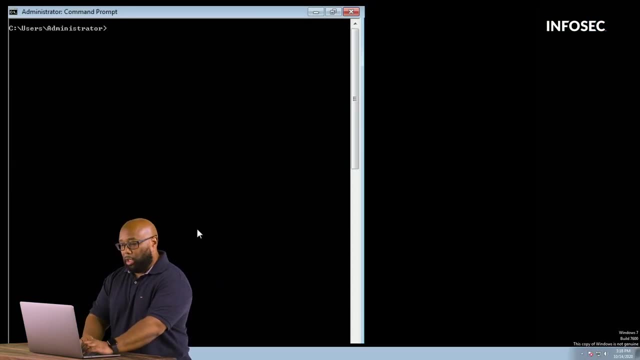 machine asking for facebook and lie to it and tell it that facebook is at my ip. let's go check the victim. see what happens now when the victim pings facebook. so victim says let's ping facebookcom and it gets pings. but look at where it says the pings are coming from 204.. so we've successfully. 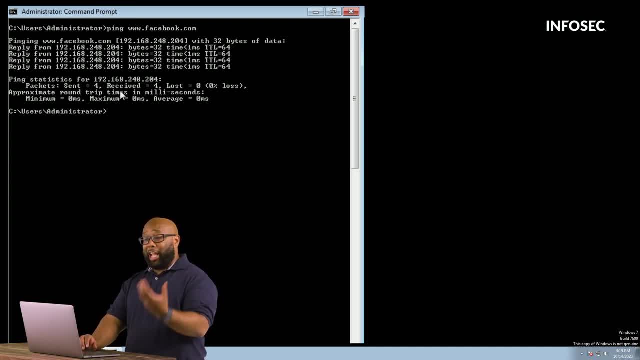 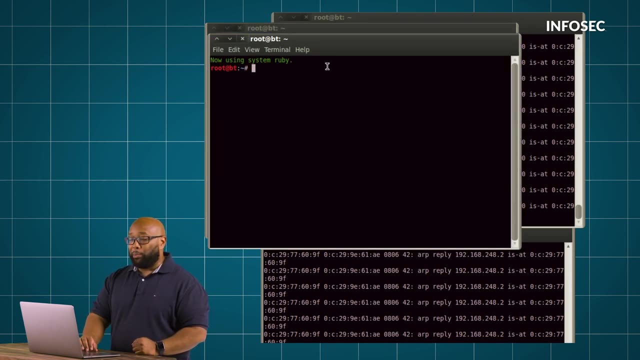 poisoned the art cache. now we've successfully dns cash poisoned them, so they can't even dns look up facebook without blindly trusting what we're telling it. facebook is. the last step of this is now. i simply need to go out and make sure i have myself a nice, clean copy of facebook that. 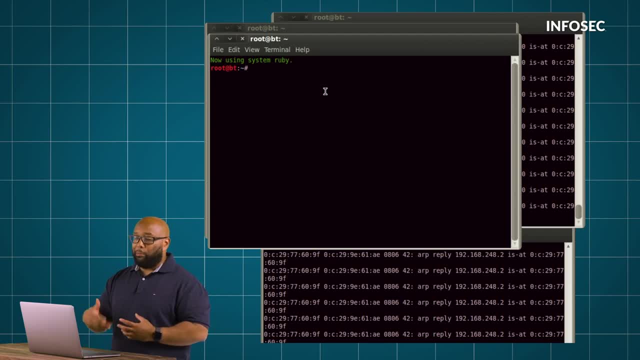 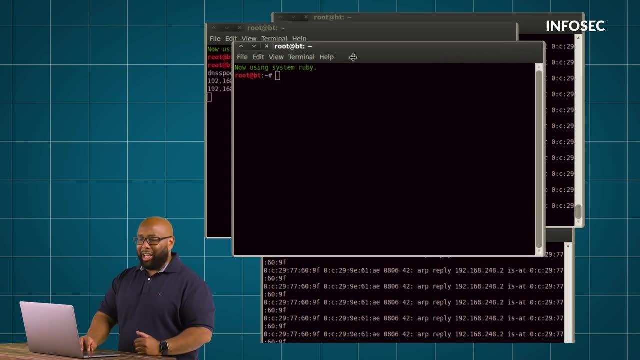 looks just like facebook but actually has malicious code in it that will give me control of that victim's machine if they are to browse to my particular copy facebook. this is also known as a client-side attack against the browser that we're going to use to do the actual exploit here. 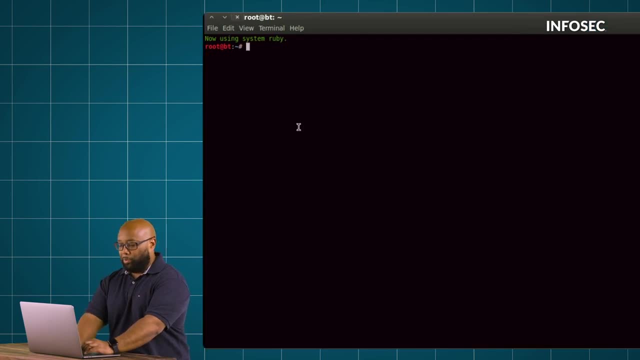 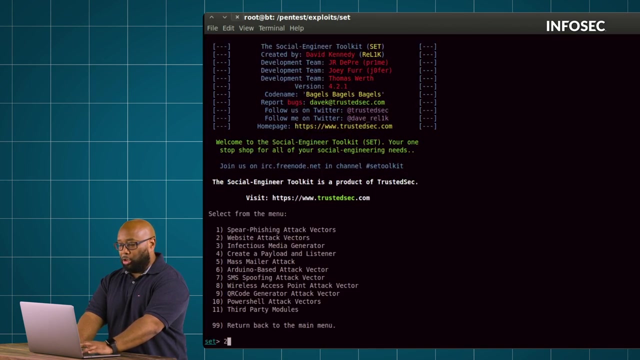 so that sounds complex. let me show you how simple it actually is. i'm going to load up a tool that's been around for a lot of years, written by dave kennedy, called the social engineers toolkit. i'm going to pick one for social engineering, two for website attack vectors. 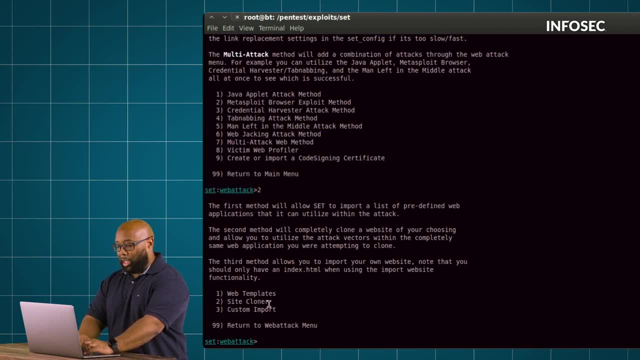 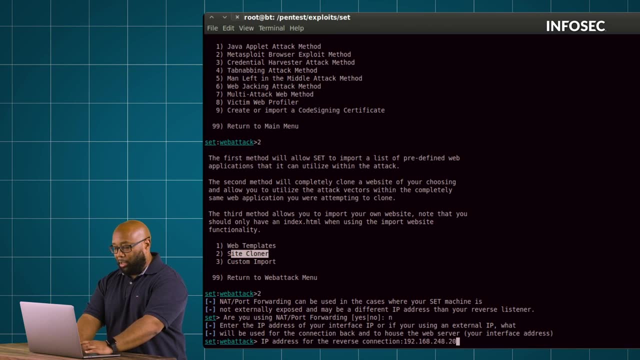 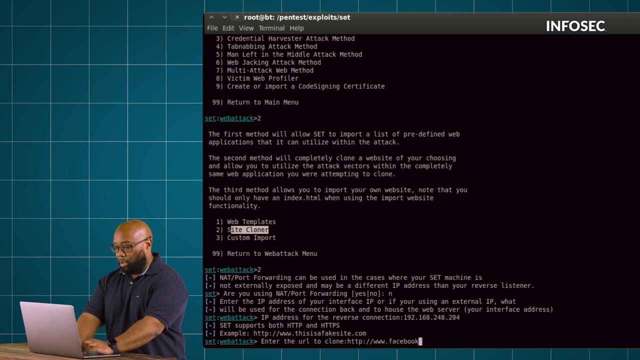 and two again for browser exploit method. i'm going to go to site cloner. i'm going to say no to natting ip. i want to come back to. that's going to be mine. who do i want to clone? let's just say facebook. and then i'm going to use browser autopawn, because these hundreds of exploits up here are basically 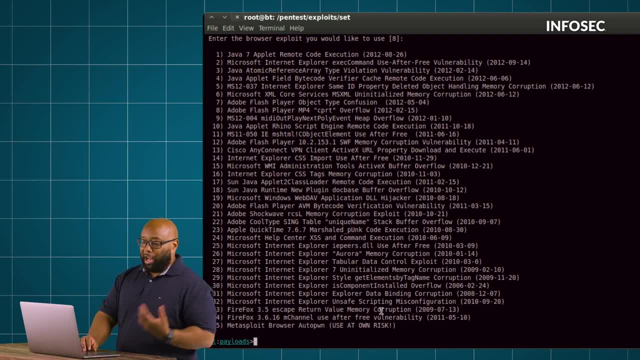 depending on me knowing which browser victims use, i don't know what browser the victim is going to have, because it could be different browser and os combinations. so i'm going to pick autopawn, which means that when the victim hits my fake facebook server, the server is going to look at. 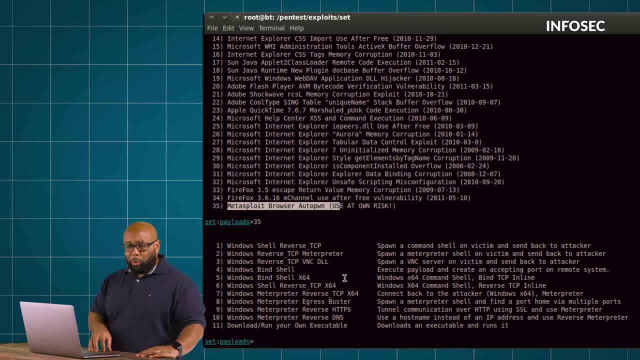 that victim's get request and decipher what the browser and os is and then send the appropriate exploit based on that. alright, i'm going to pick meterpreter as my payload. in other words, if i'm able to export the machine, what do you want to get as your loot? 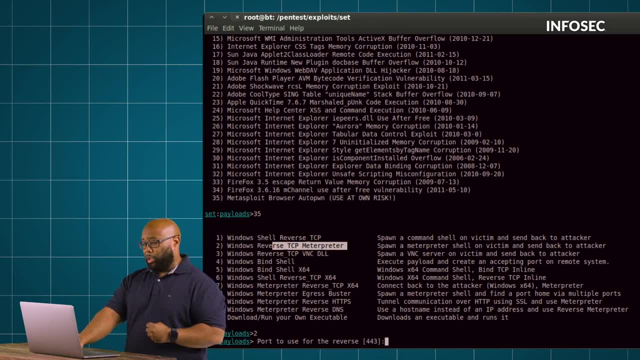 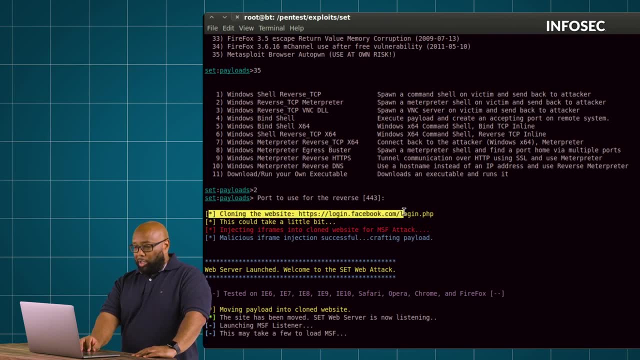 i want a meterpreter session so that i can take over the machine. let the port stay 443, and now it's off to the races. it's going out. it's going to the default facebook login page. as you can see, there it's cloning that, which means it's copying it down. 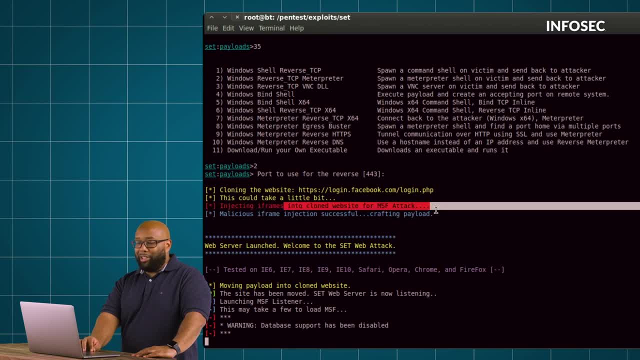 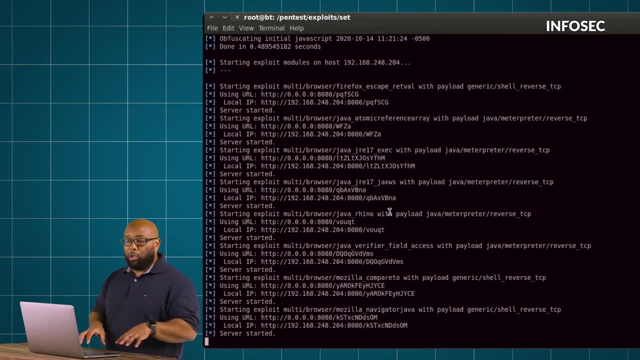 now that the lever is open, Now it's putting the malicious code that I've crafted inside that fake Facebook copy And now it's standing up a version of the exploit for every possible browser and operating system combination and storing them at a slightly different URL on my server. 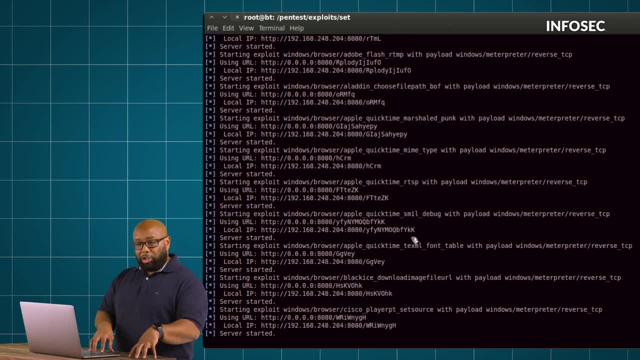 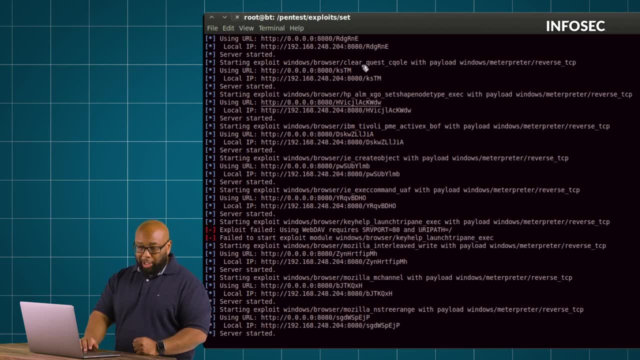 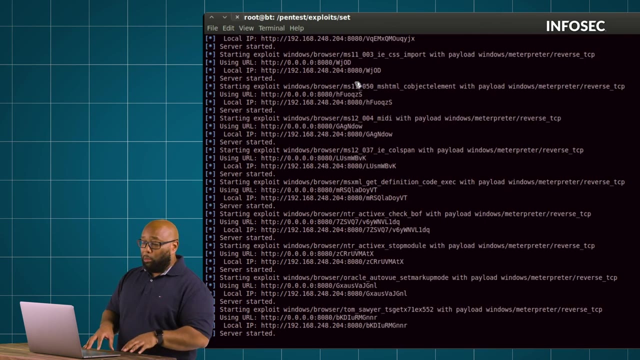 So when your browser hits this server, it's going to look at your browser version, look at your OS version and then simply send the appropriate exploit based on that, which we're loading them all right here. Once this is finished, the only thing we have left to do is go play victim and see what. 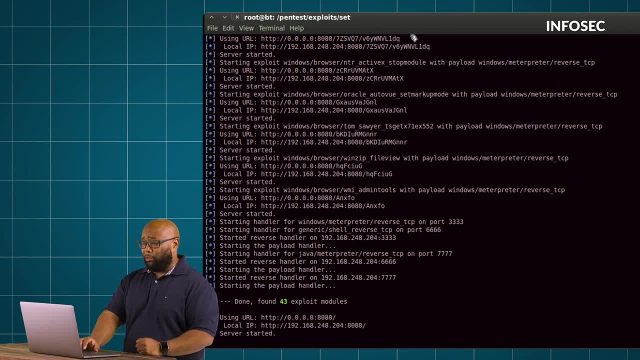 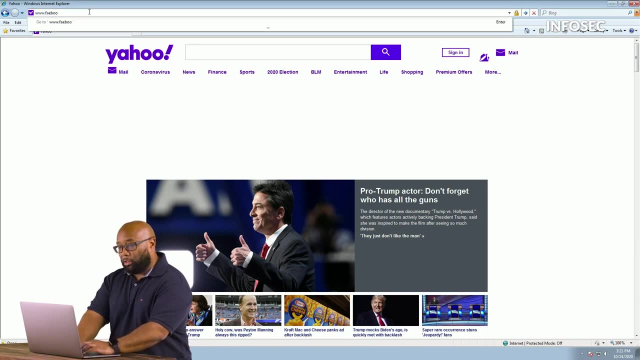 happens when the victim simply does what the victim does every day and tries to go to Facebook. So we jump over, go to the victim, We open our browser, We load facebookcom in there, our browser, And at that point, right there, it's game over. 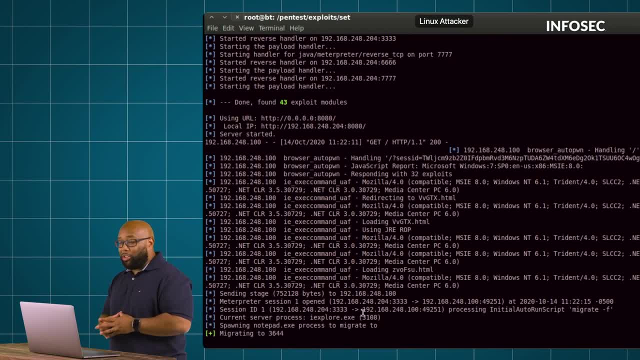 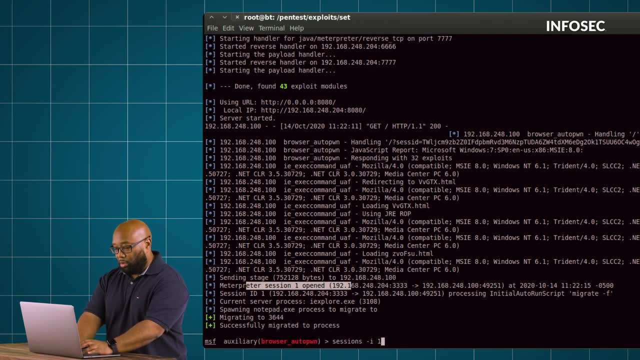 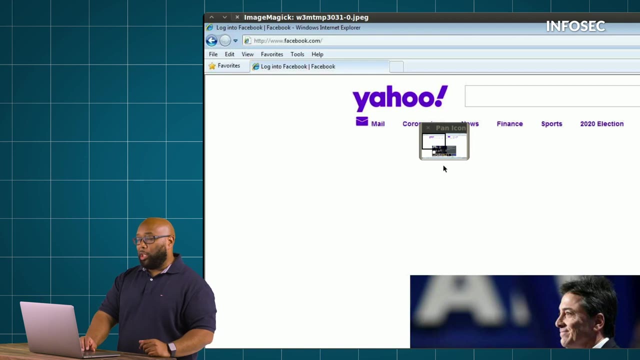 We go back and look What you see happening on the attack. Our side is, the attacker now has a session. We connect to that session as the attacker. Take our obligatory screenshot here to prove that we have it And at that point we own that machine. 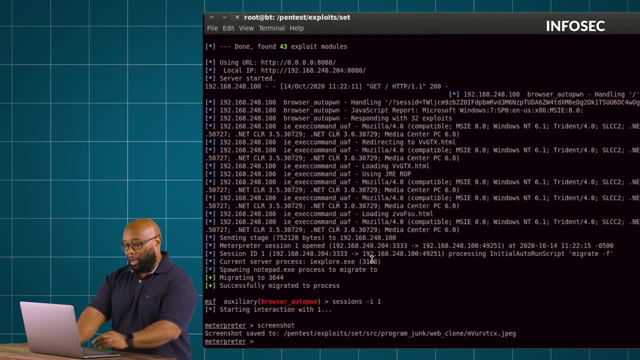 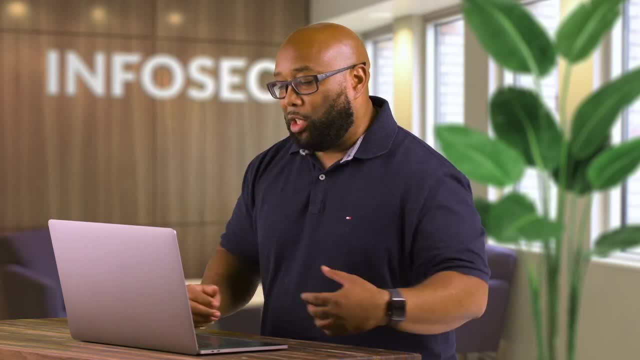 It belongs to us completely. It's no longer that victims, It is ours. We can drop into a shell and it's all game over at that point. And that, folks, is what a man in the middle attack looks like. And now you can see.